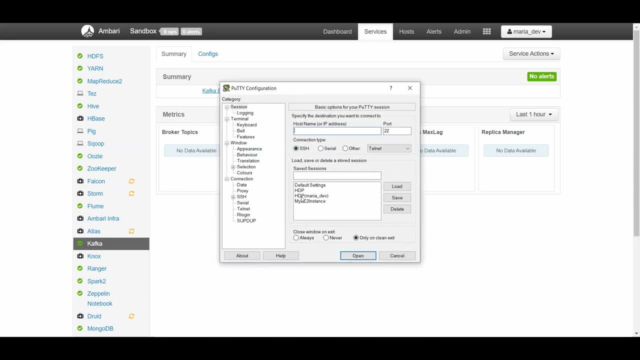 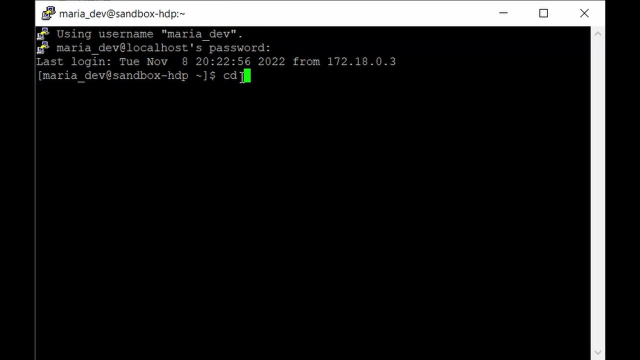 step would be just go to the PuTTY and login as Maria underscore Dev. So you know the password. So the first step would be to go to the Kafka directory. So, as you already know, the Kafka directory lies in user sdp slash, current slash Kafka broker. So here, 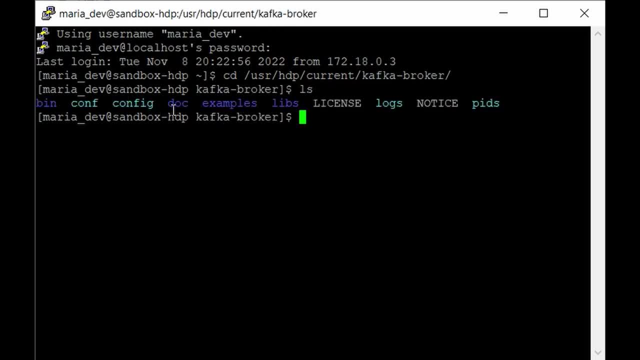 we have all the directories like bin, conf, config file, as well as the logs directory. So here you have to go to the configuration directory now. So go to configuration directory and go to configuration directory and go to Kafka directory. So here you have to go to. 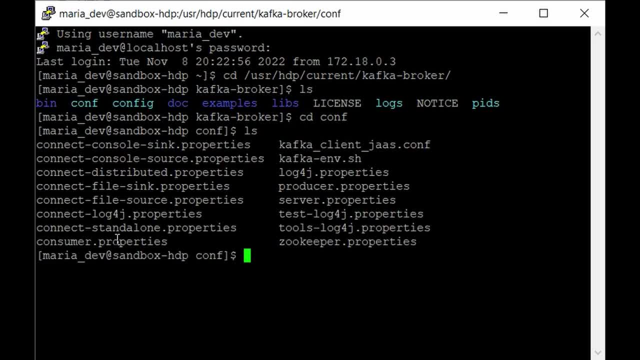 conf and in this directory you will find the consumer consumer standalone properties which we are going to use it to make the connection to our weblogs, text file which we will download from the github and connect to a kafka topic. so we will need this file and also we have the sync. 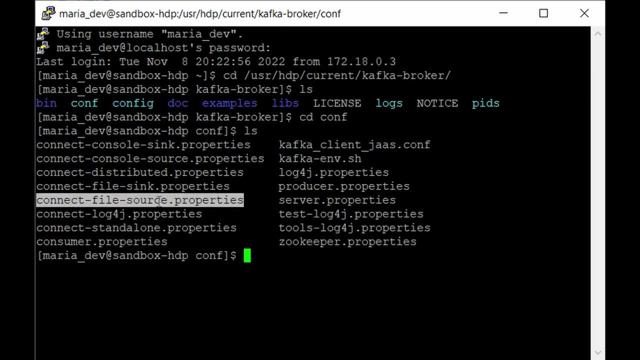 the connect file syncproperties and the connect file sourceproperties. so in this properties we will set the paths for our source as well as sync. and also we need to define the kafka topic here. that means we need to make some modification in these three files, but since this is kafka, 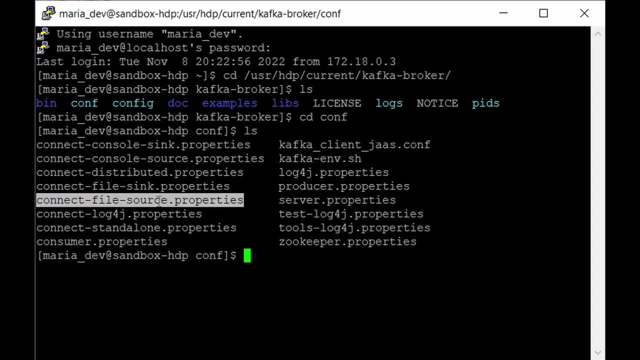 directory and we don't want to mess up with our kafka installation. we can copy these files to our home directory and then we can modify it. so for that purpose we'll use the copy command. so just give like cp, then we'll copy this file. so just take the standalone properties file. 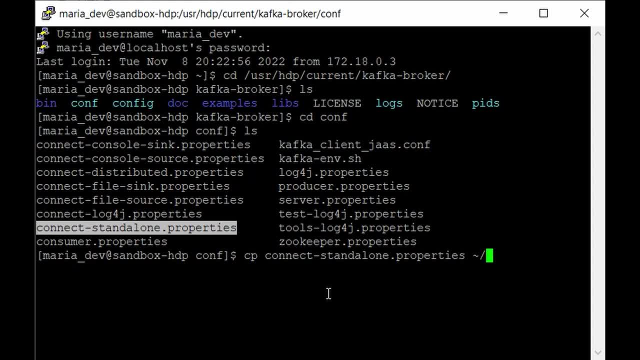 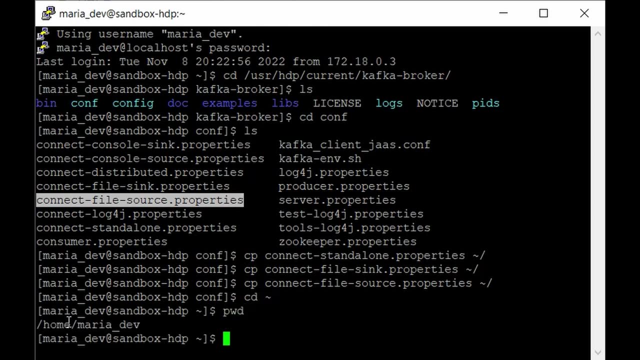 and we will paste it in the tilde home directory. after that we'll also get the sync in the home directory as well, and at the last we'll get the source file. that's it. so we'll go to the home directory now. so, cd tilde. so if you give present directory, we are in the home. maria dev directory. 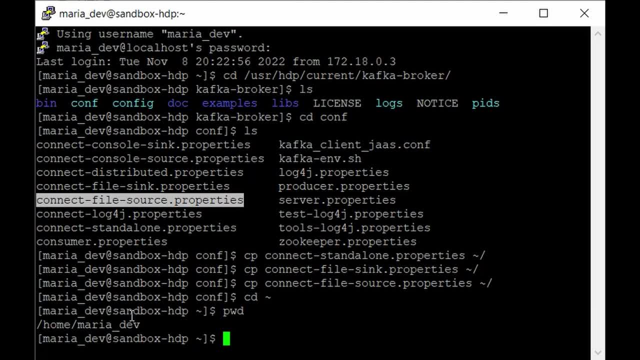 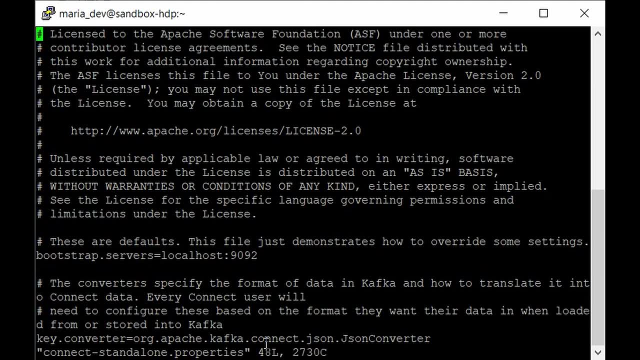 now. so here we can use the vi editor to edit some properties in these three files. so the first file is connect standalone properties. yeah, so here we need to change bootstrap server and make it listen to the open port, which is six, six, six, seven, which we have seen in the previous lecture. so just 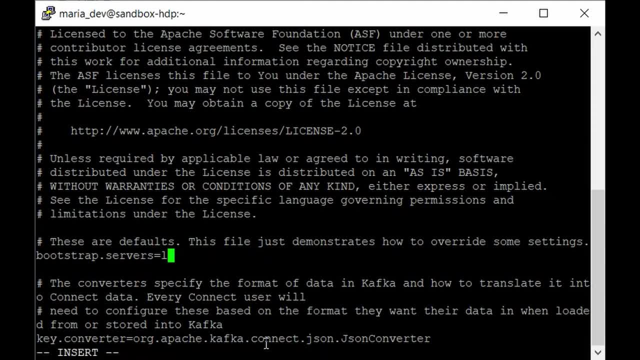 go to that path and hit i to insert mode. just remove it and give the host name as sandbox: hortonworkscom. colon six, six, six, seven. that's it. that's all you have to do. so just hit escape to get back from the edit mode and give like colon wq and enter to save that file and do the same. 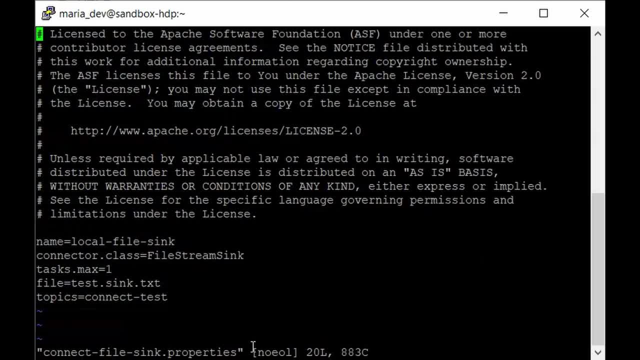 for the next file, which is syncproperties. just open this file and here you need to make changes in the file and the topic. so in here just go to the file, hit i to enter into edit mode and change the file name as give the path for the home directory. so give like home slash. mary underscore. 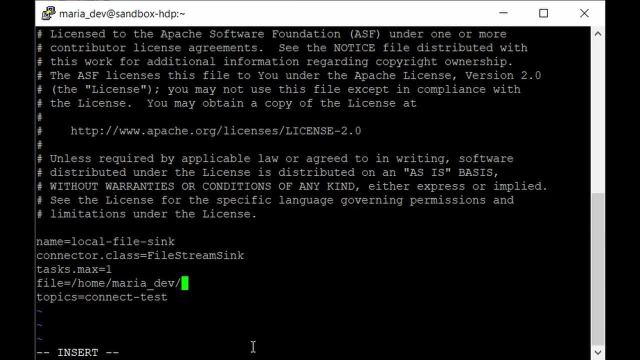 dev slash and our file name will give like logouttxt. so this is the same for our file. so we will read all the data, or we can say event streams from our source file, then write it on the kafka topic and then this is how we do it. 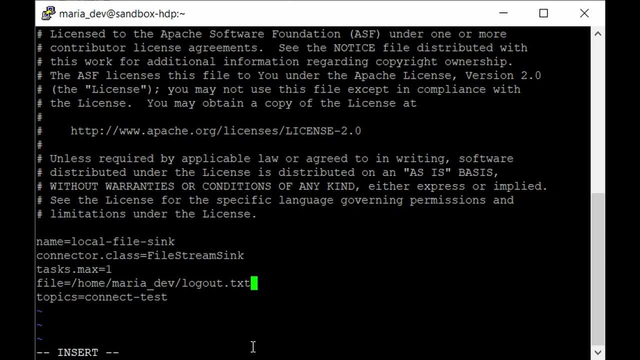 again write it back to the consumer in our logout dot txt file and on the next line you have to also mention the topic name. so again, just go into insert and change the topics. as we can give anything so we'll give like log dash test. so i guess we are done here, so just escape and our 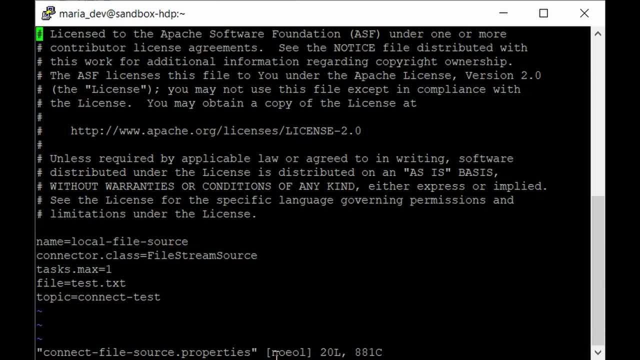 last file is source dot properties. go into that, and here you have to again change the file name. so here our file name will give it as access underscore: lock dot txt. so this is the file which we'll be going to download from our github repository and on the next line again give. 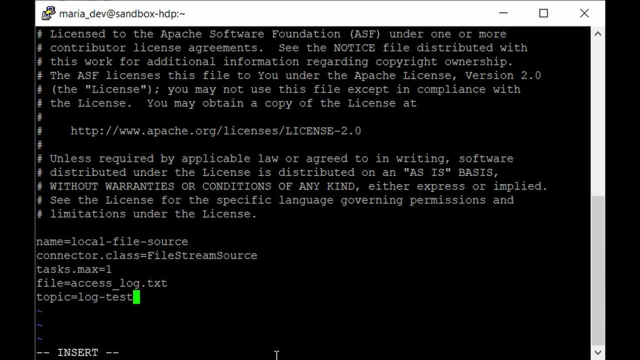 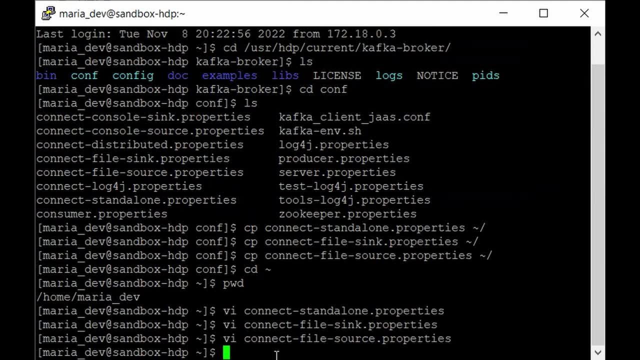 the same topic, which is log dash test. that's it. we're done here, get out from here and we're good to go. we just need to download that file. so you know the command right. so just give like: wget https colon slash, slash, raw dot, github usercontent dot com, the username slash. 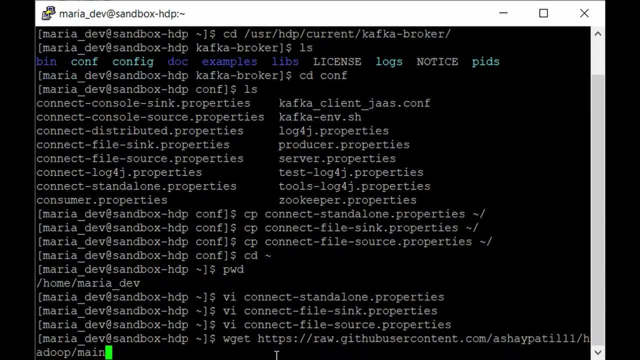 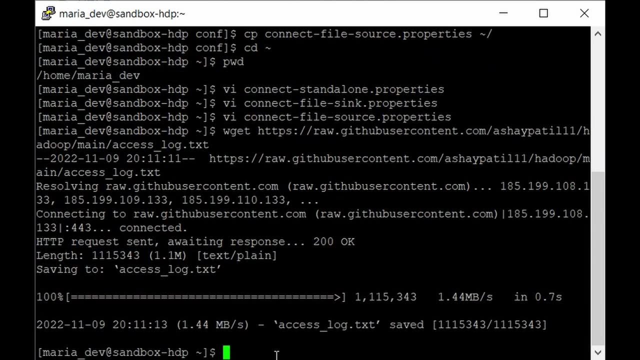 11: slash hadoop. slash main, which is the branch name. slash access underscore: lock dot txt. so this is our log file which we're going to use as a source file. so just hit enter and that's it. we got the file right. so if you give ls, you will have the access log dot txt. 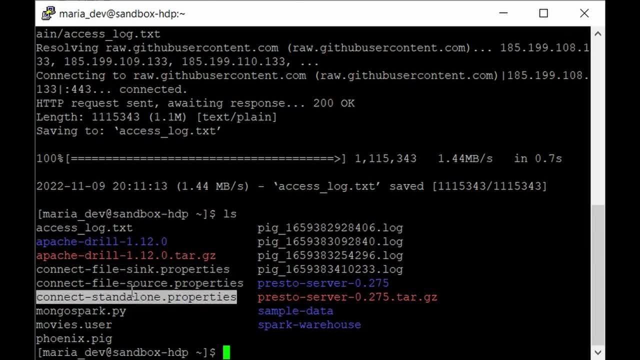 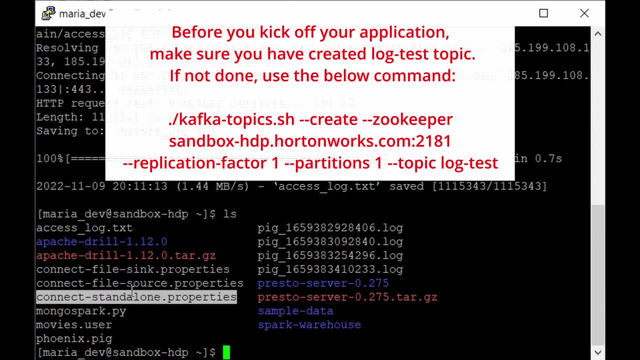 sync source and the standalone properties file. so you're all set to kick off your real-time streaming application. so the first step would be you need to go to again to the bin directory and kick off your consumer. so to do that, just again, give to cd user sdp, current kafka broker, slash bin. so in this bin directory you need to kick off. 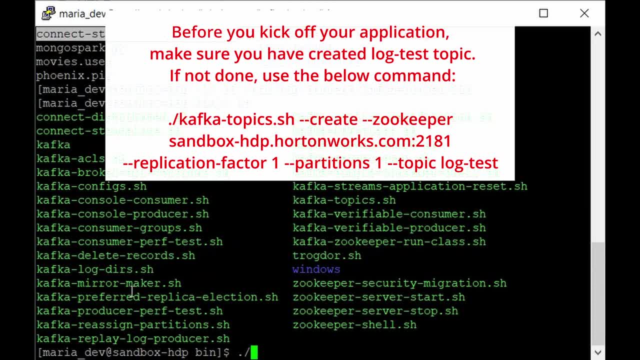 the kafka consumer file. so just go dot slash kafka console dot dash consumer dot sh. then you have to go to the msg file and then you have to give the access log, dot txt, and then you have to click on the address to zookeeper. so give like zookeeper on the localhost colon 2181. so this is the port for. 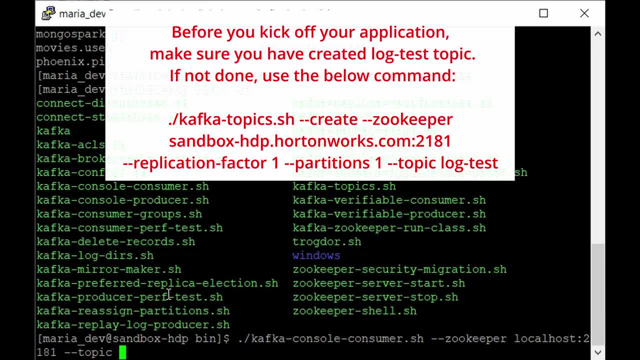 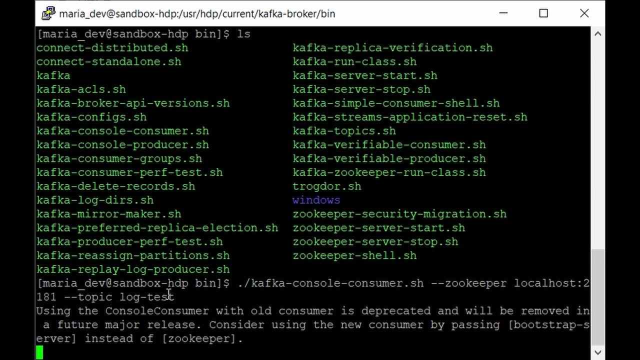 zookeeper and the topic name. so our topic name is log dash test. as we have mentioned, we know both source and sync, so log test, that's it. if everything looks good, hit enter and that's it. so your consumer is going to listen to any changes in your log file. so now you have to kick off. 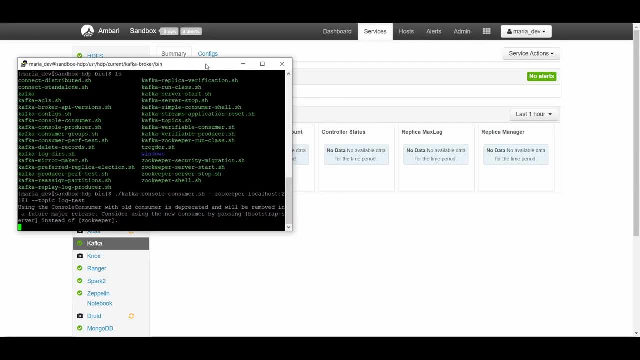 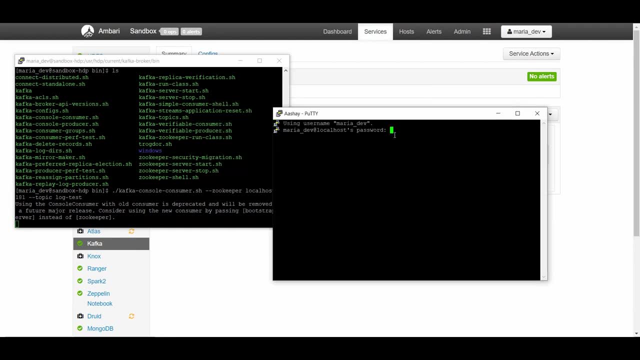 the new terminal now. so the next step would be: just here is your consumer running and just kick off the new putty terminal. so again, login as a maria underscore dev, and here again you have to go to the bin directory. so just go to cd user sdp- current kafka broker, slash bin, and here you need. 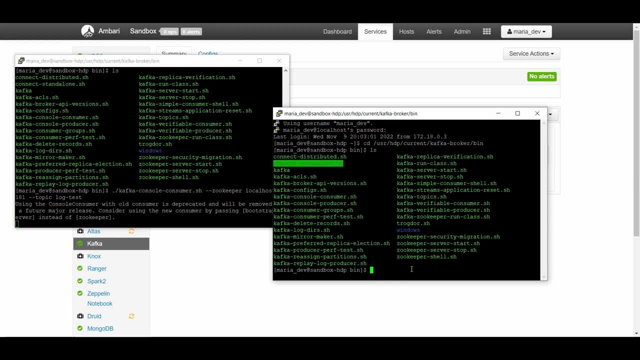 to kick off your connect standalone dot sh file. so just give like dot slash, connect standalone dot sh and you have to pass all the properties file which is connect standalone dot properties, which is present in the home directory. then we have the source and the sync properties file, which are also present in the home directory. so that will go as. 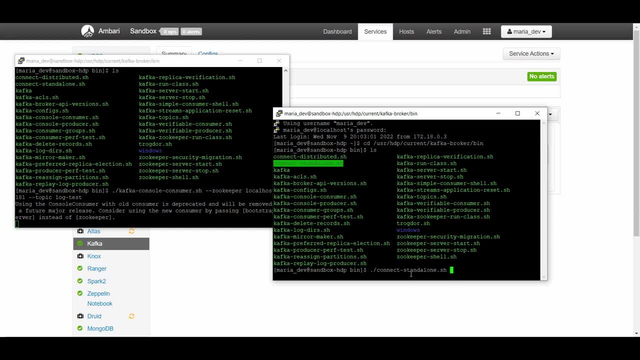 an argument for this file. so to do that, just give, like path path which is tilde slash, the name which is connect dash, standalone dot properties. then again give the source, which is connect dash file. so that's it. so if everything looks good, just kick off. so this will take about a second or so. 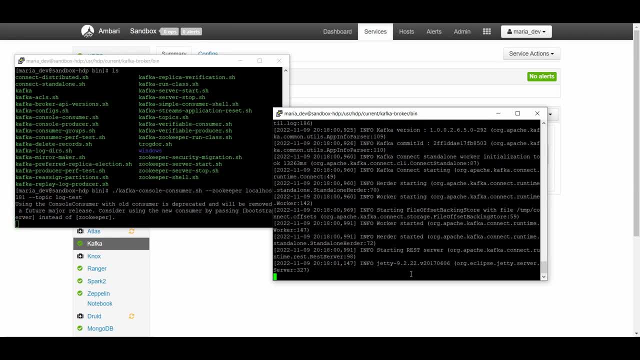 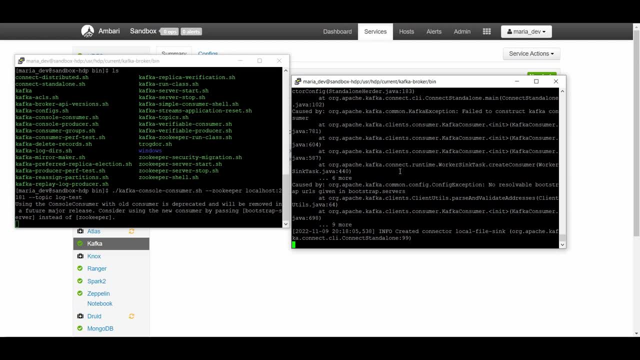 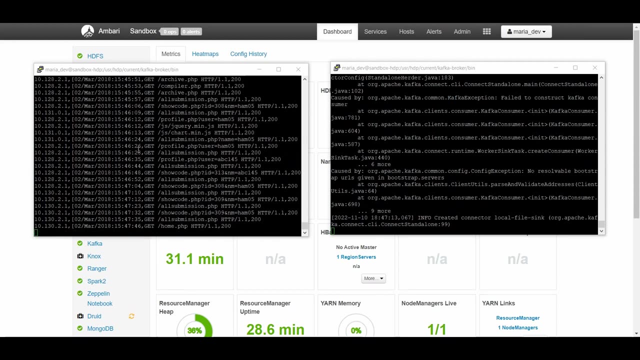 to connect to kafka so it is running now. so, if everything is fine, it will pick the data from our access logtxt and publish it to our kafka topic. so, as you can see, all the logs from access underscore logtxt file have been published to our log test topic. so this was. 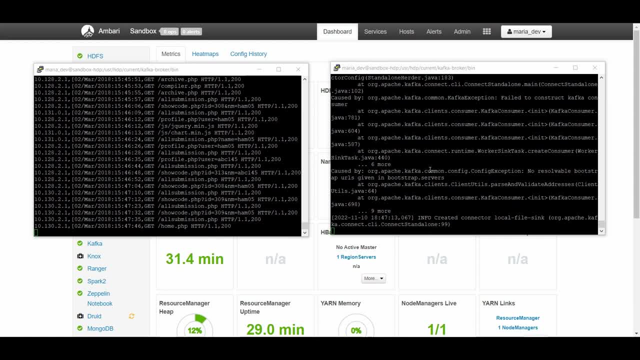 a real time. so what we have done is we have built a real time streaming application where we have set up all our properties file, where we have defined sync dot properties, which has the target file and the topic, and the source, source dot properties, which has the source, which is nothing. 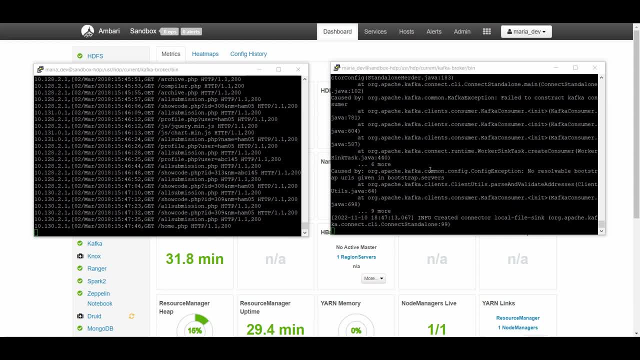 but our access log file which we got from kaggle and the topic, which is again the same one, which is log test, and all the data from access log file have been published to our kafka topic. so i hope you got a clear idea how kafka works under the hood and how it publishes records in real time. 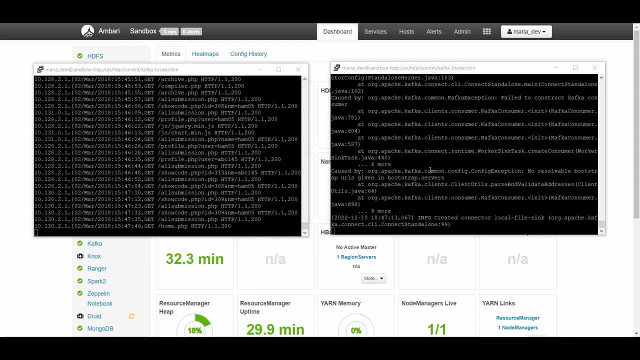 on a topic and then we can build a consumer application to further process that data down to get meaning out of it. so this was just a simple tutorial for your understanding around kafka and you can also explore more when we will cover kafka in detail in our upcoming tutorials. so if you have 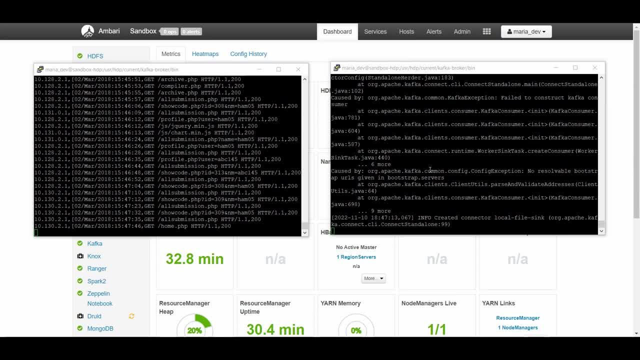 any doubt in this, just let me know in the comments and i'll get back to you as soon as possible. i hope you like this video. if you are new to this channel, make sure to subscribe to the channel if you are new to this channel, and i will see you in the next one. so till then, bye, bye, have a great day.